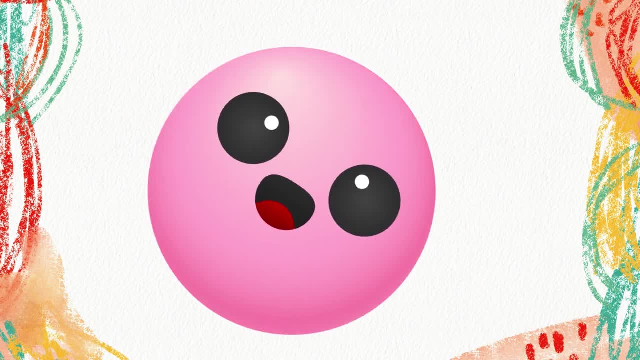 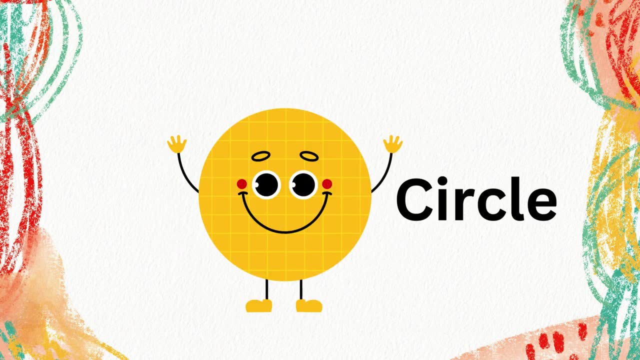 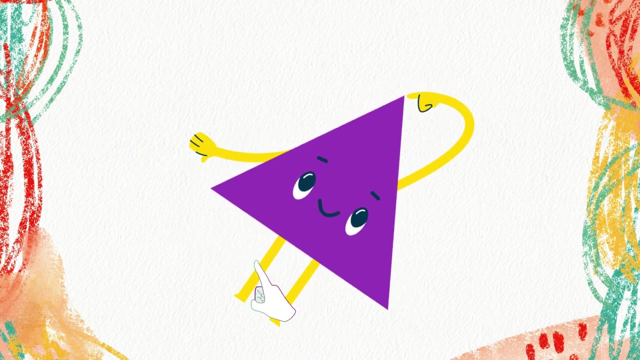 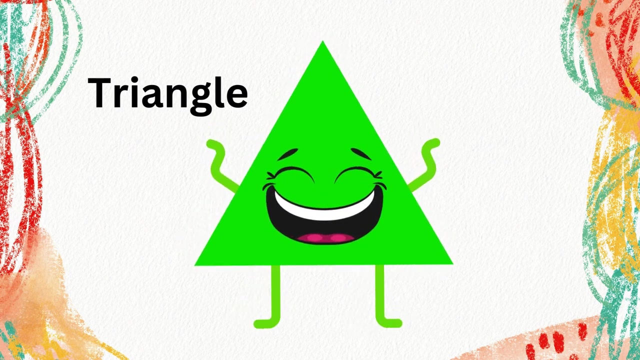 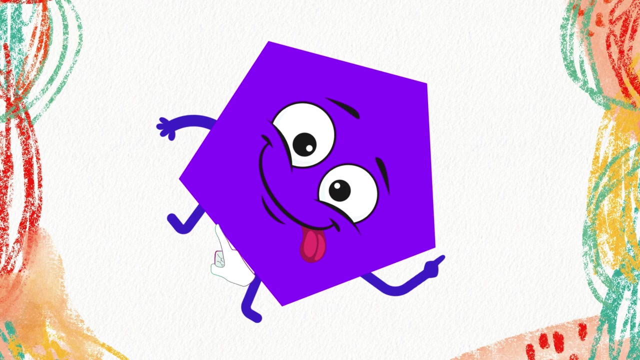 I am a shape. I like to roll and roll and roll. What am I? A circle, Great job. I am a shape I have three equal sides. What am I? Yes, a triangle. I am a shape I have five sides. And guess who I am? Yes, great job. 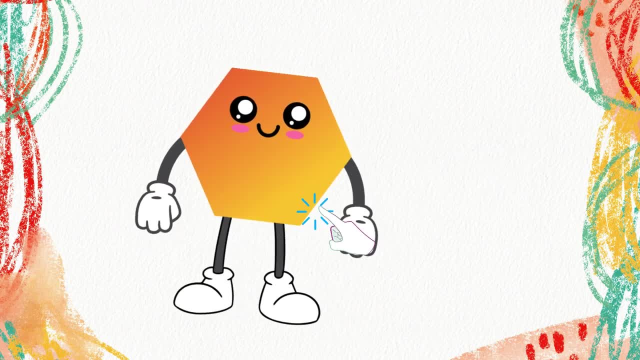 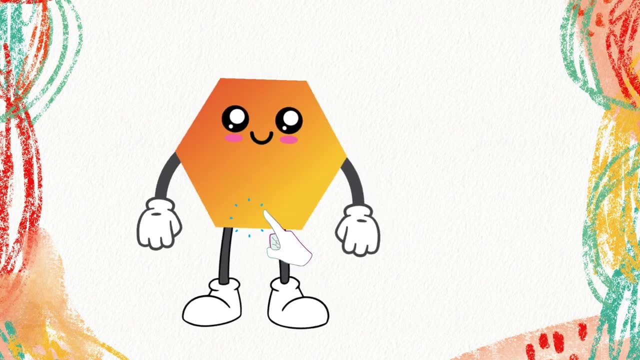 I am a pentagon. I am a shape. I have six equal sides. What am I? Yes, a triangle. Yes, a triangle. I am a shape. I have three equal sides. What am I? Yes, a triangle. 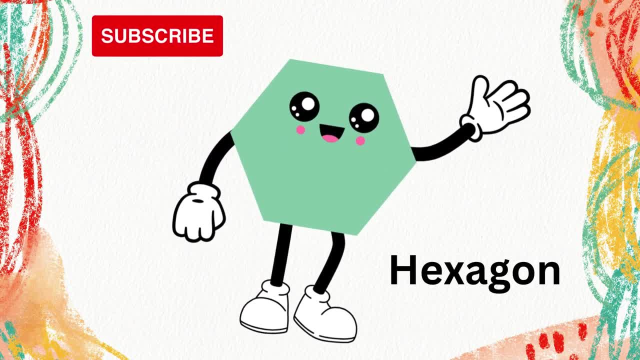 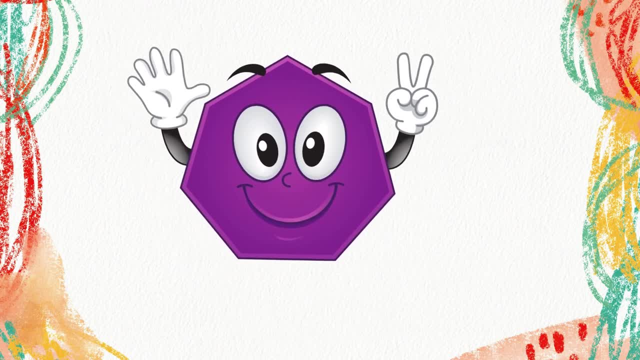 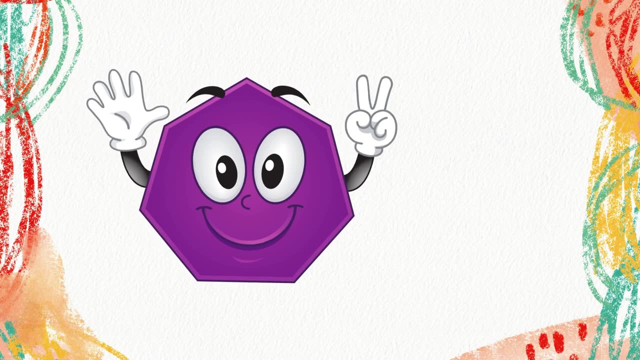 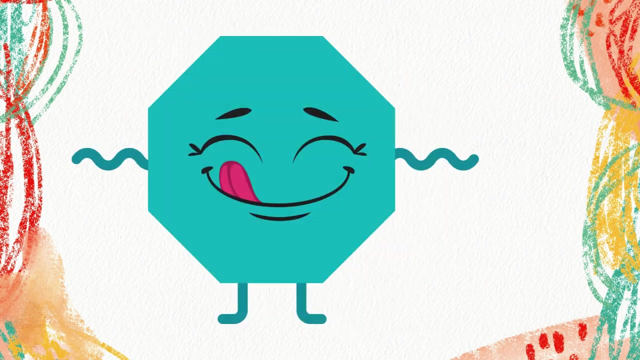 Yes, a hexagon. Great job. I am a shape. I have seven equal sides. What do you think I am Great job. Yes, you're correct, I'm a heptagon. I am a shape. I have eight equal sides. What am I? Yes, an octagon, Great job. 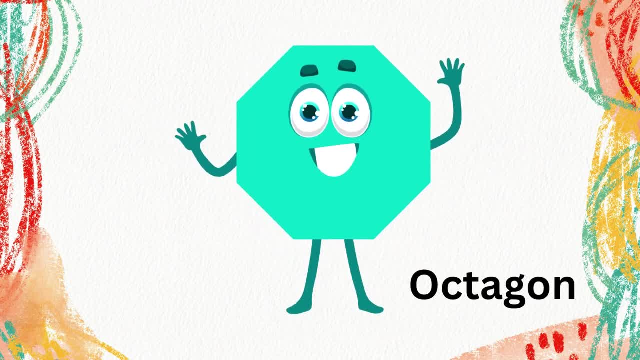 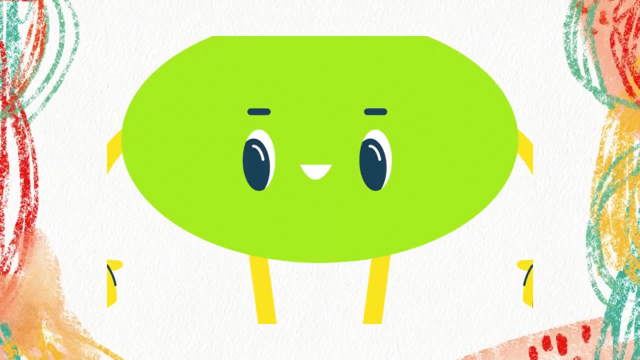 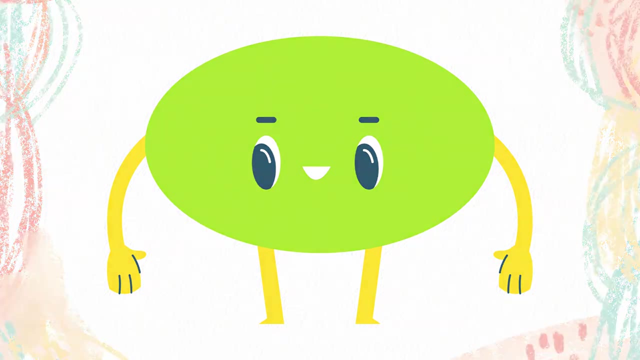 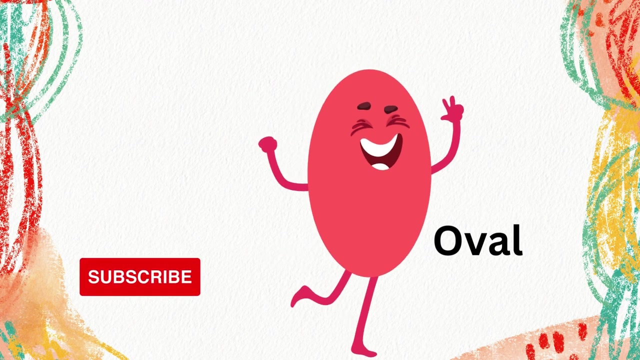 Now I look like something you've seen before, like a circle, But I look a little bit longer. What do you think I am? Yes, I am called oval. Great job. I have two flat sides and two round sides. What do you think I am? 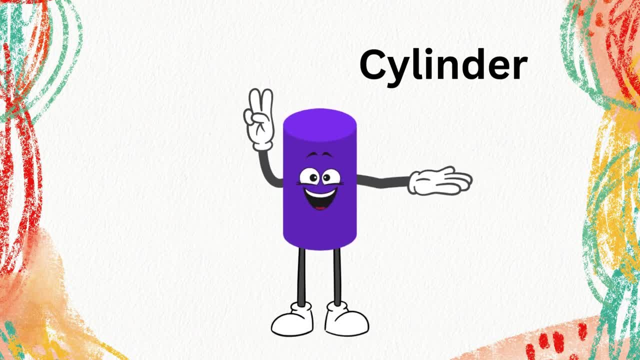 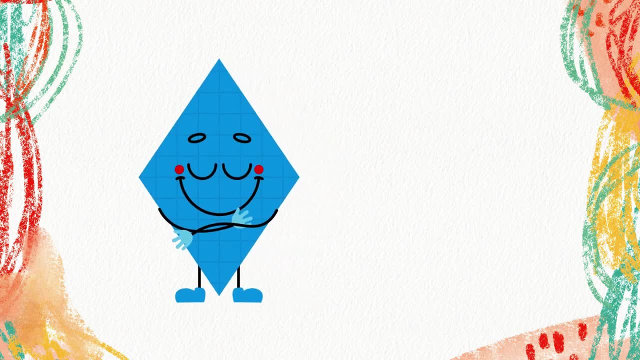 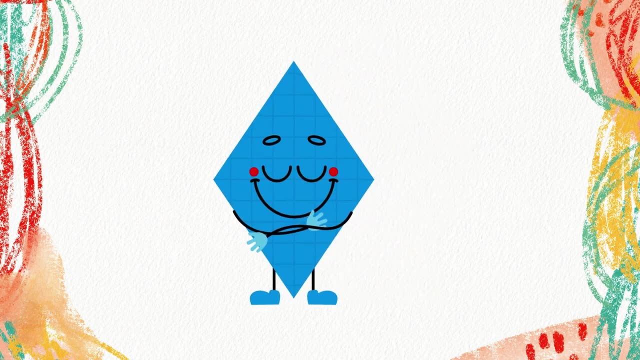 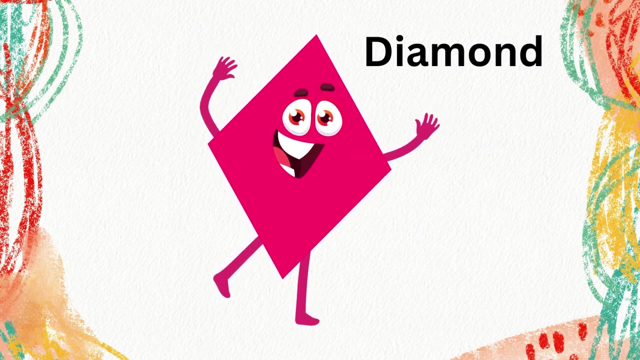 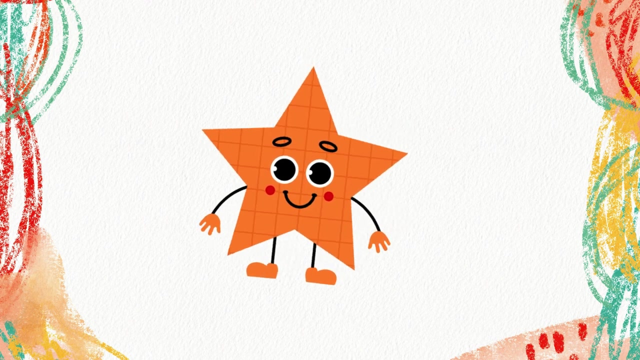 Yes, I am a cylinder. I am a sparkly shape with four sides that are all the same height. What am I? Yes, a diamond. I have five points And you can see me all in the sky. What am I? Yes, I am a star. 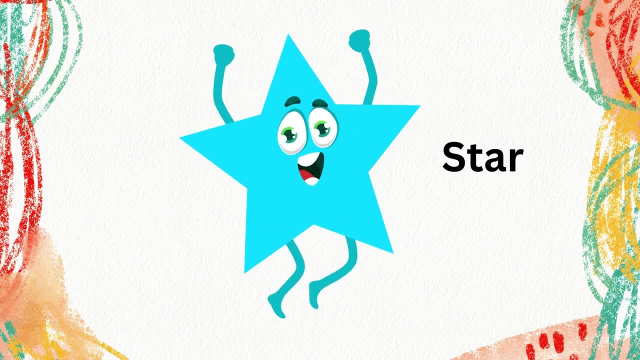 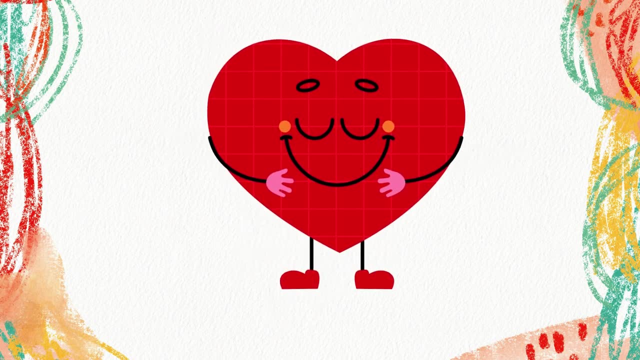 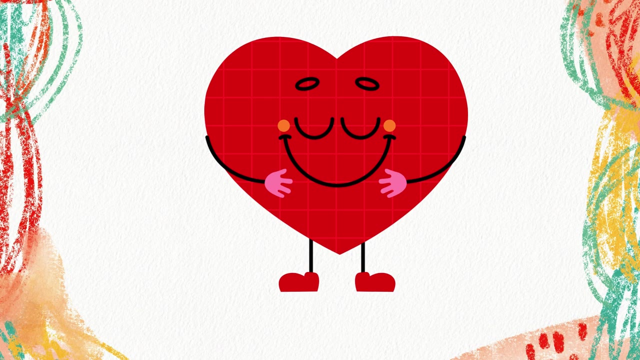 Well done. I am a special shape that looks like two round humps at the top and a pointy V shape at the bottom, Like the symbol of love. What am I? Yes, I am a heart. Yes, I am a heart.